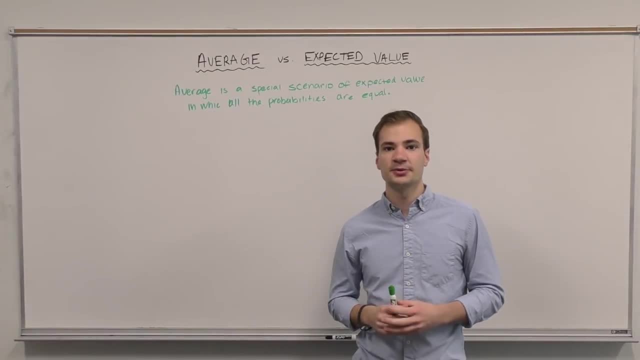 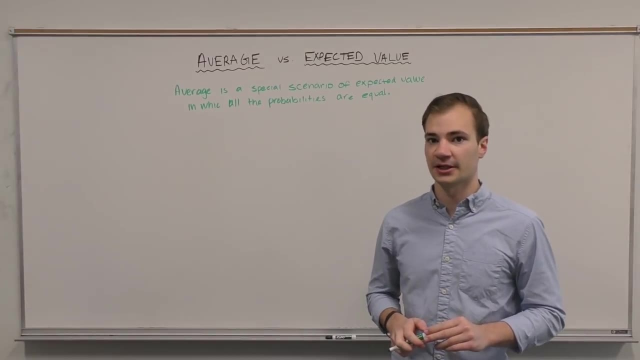 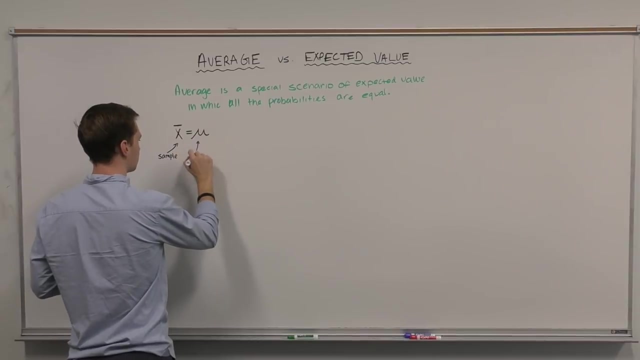 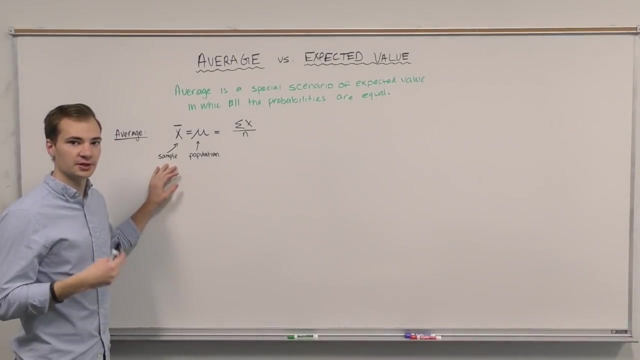 ticket is actually less than its cost. Now let's get into a little bit of the math behind it. The formula for average is as this: Where we use x-bar when we're talking about a discrete sample, and a mu to represent the average of a population as a whole. 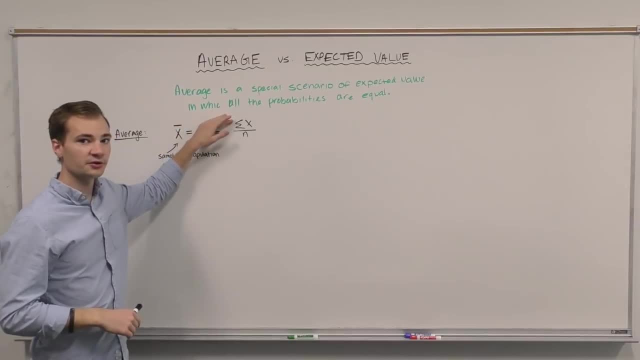 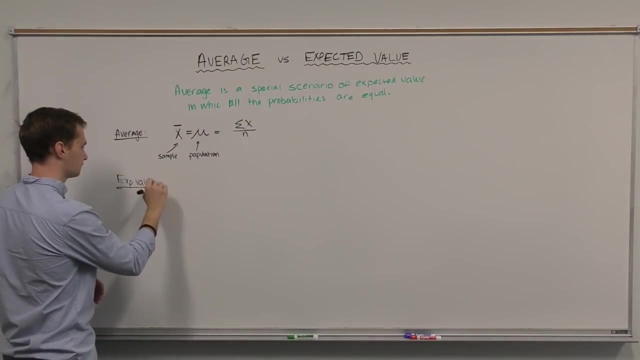 And this is a formula you're probably very familiar with. It's the sum of all of our factors, The number of values divided by the number of values we have. Now let's look at expected value. Let's break this down. This is called the expectation of x. 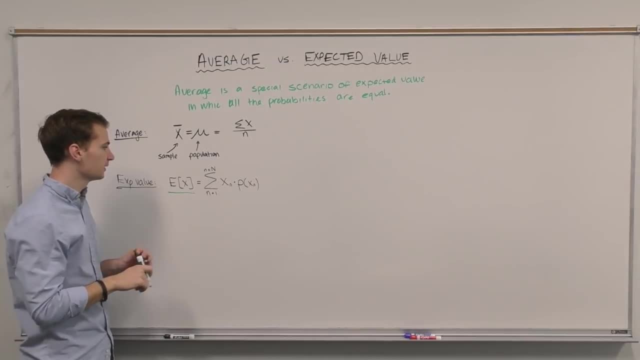 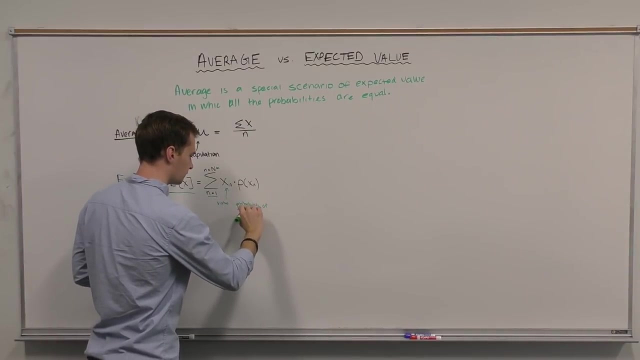 X is our random variable. You don't need to know about that, but it's the same x that we represent up here Now. it's the summation beginning at n equals one And going until sum number n of our value times the probability of that value occurring. 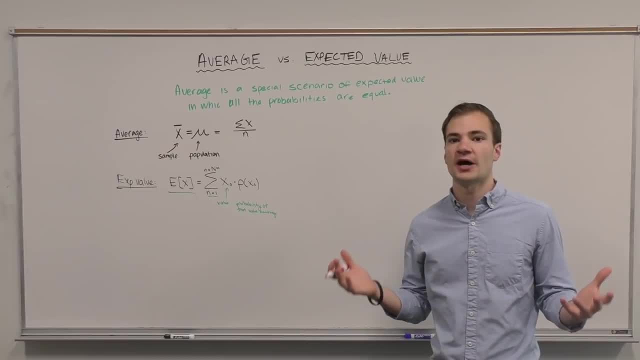 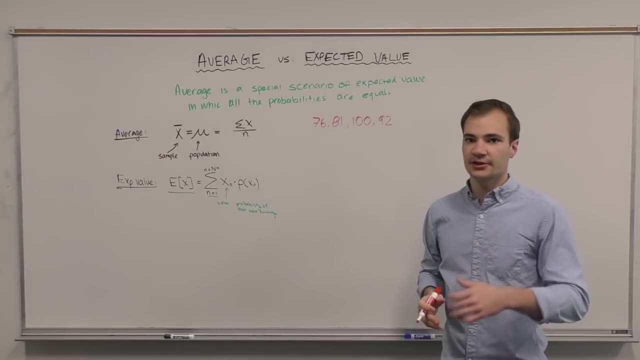 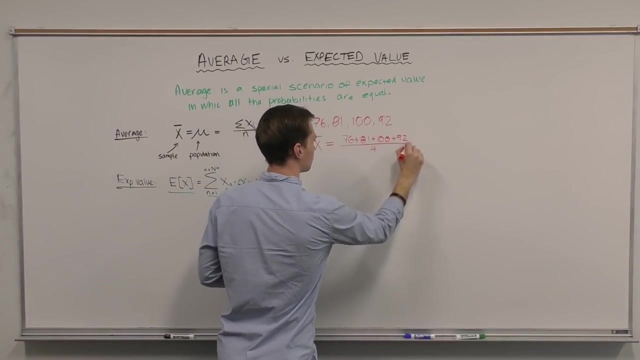 Let's look at an example of students who scored a certain value on their tests. Now let's calculate our average. We're going to calculate our average. We're going to calculate our average. Again, this is something you should be pretty familiar with. 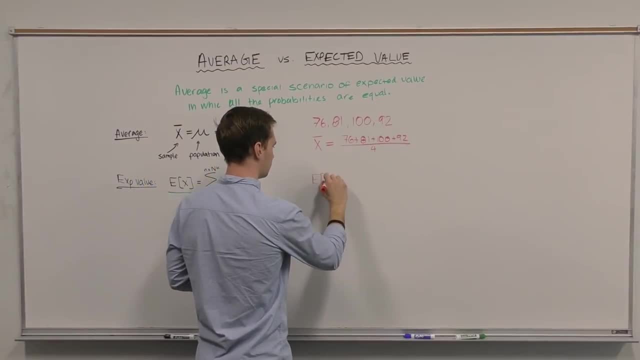 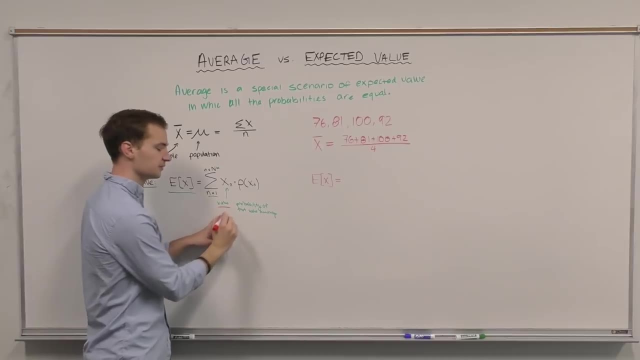 Let's look at expected value now. The x values of this part are easy to think of. We know that the x represents the value itself, which will be these four numbers. Now, the probability of x in this scenario is if we put each one of these numbers on. 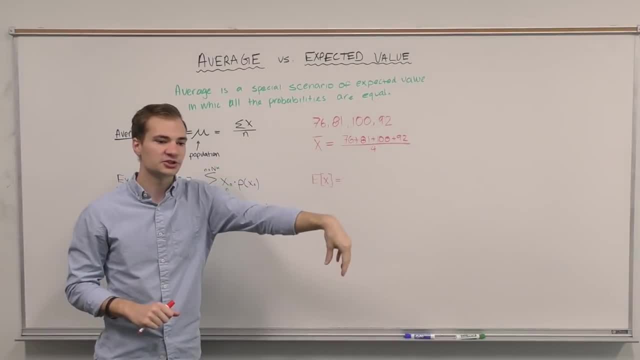 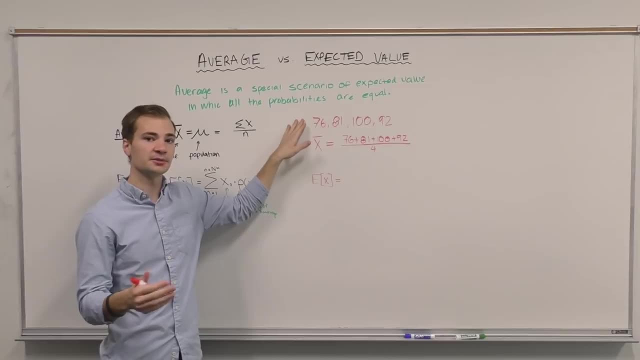 a piece of paper and threw it into a bag and I reached in and randomly picked one out. I would have a one in four chance of picking one of these. There's four of them and I have an equal probability of pulling each one. 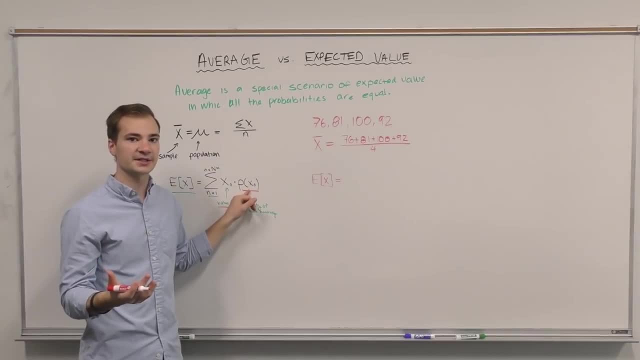 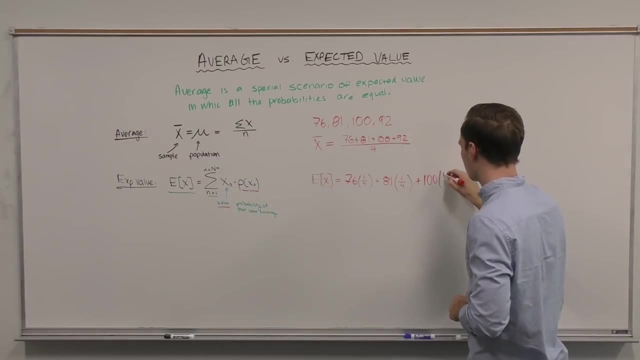 So we know that the probability of a given x is one fourth. Now I hope the gears are turning. Let's take both of these formulas. Let's look at the equation. Let's look at the equation. Let's look at the equation. 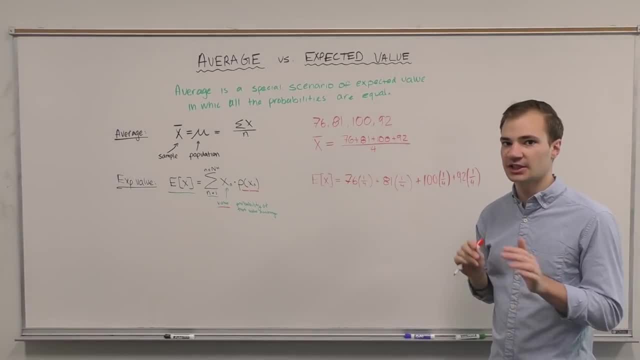 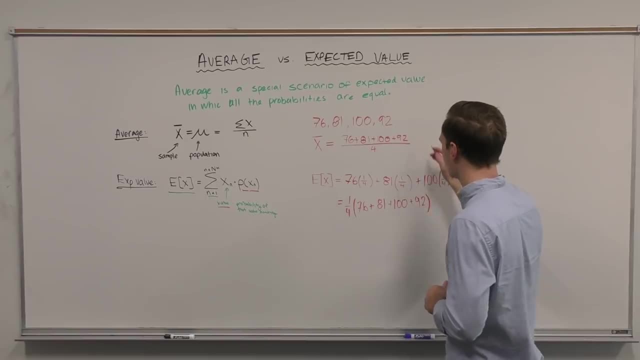 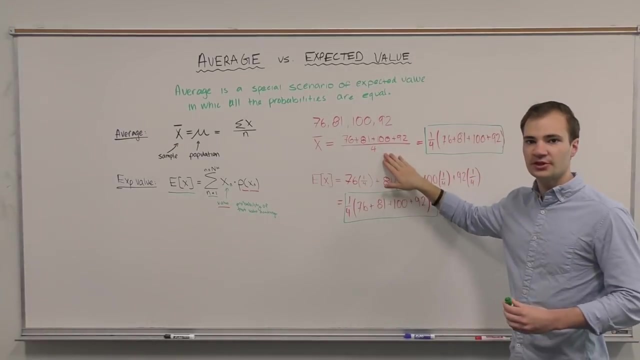 So let's do a little bit of math, a little bit of factoring, and check out what we get, And we see we get the same number. What we did here is pull the one quarter out from the bottom and bring it out front. 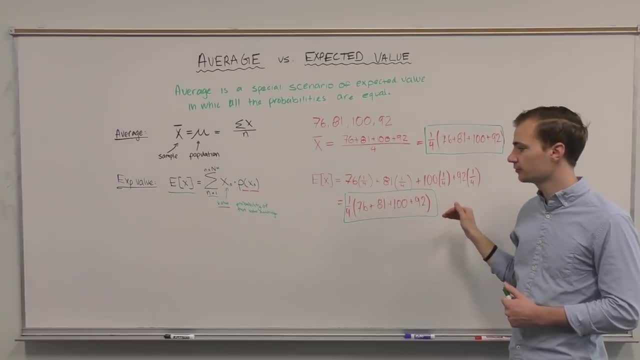 Similarly, Here we factored out a 1 quarter from each of our terms and pulled it up front, and we see that these two values are equal. Now, remember, there is an equal probability of pulling each one of these values, and that's why expected value is equal to average. 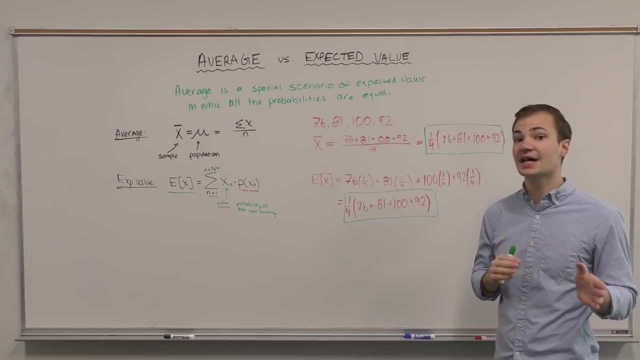 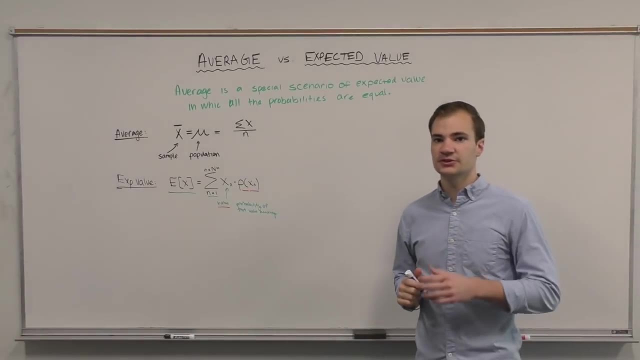 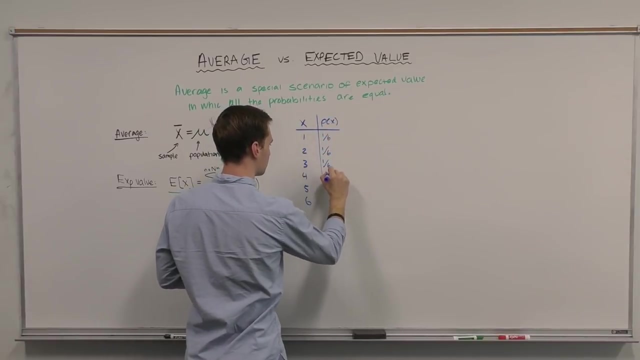 Let's look at an example now where the expected value is not equal to the average. It's a little bit more interesting If you've seen some of my other videos before, you know. I like to look at the example of rolling one die. Normally, a normal die would have this distribution. 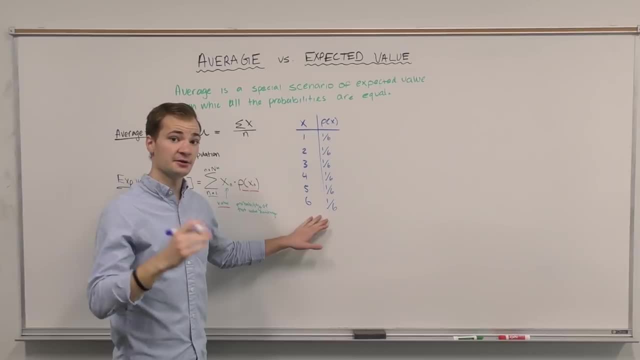 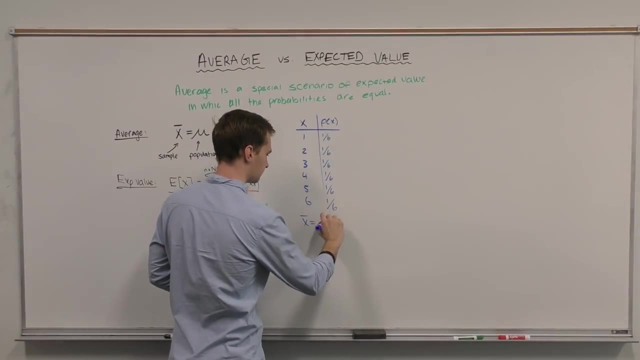 We have a 1 in 6 chance of rolling any of these values. The average for this is fairly easy to calculate. We can almost do it in our heads. The sum of all our values divided by the total value of the die is equal to the average. 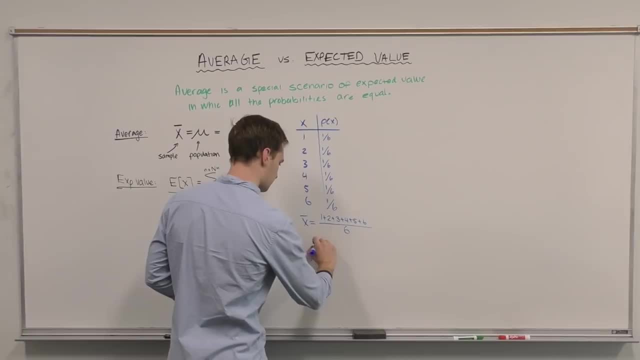 The average for this is fairly easy to calculate. We can almost do it in our heads. The sum of all our values divided by the total value of the die is equal to the average. The average value divided by the total value of the die is equal to the average. 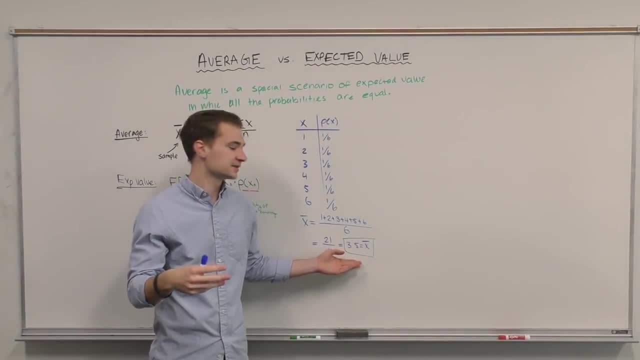 So the average value, if I rolled a 1000 dies, would be a 3.5. And this is pretty easy to see on something like excel. Now what if we transform this so that it was not an equal die? In other words, a 5 and a 6 were more likely to land than a 1,, 2, 3 or 4.. 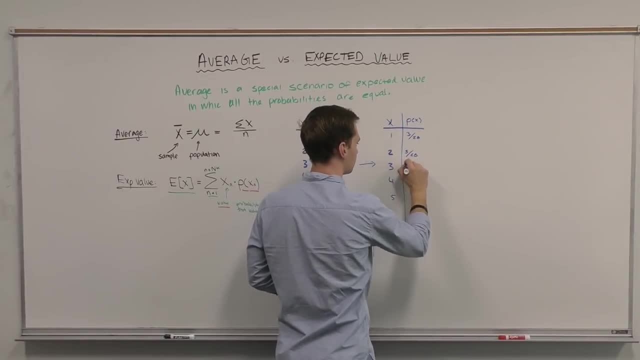 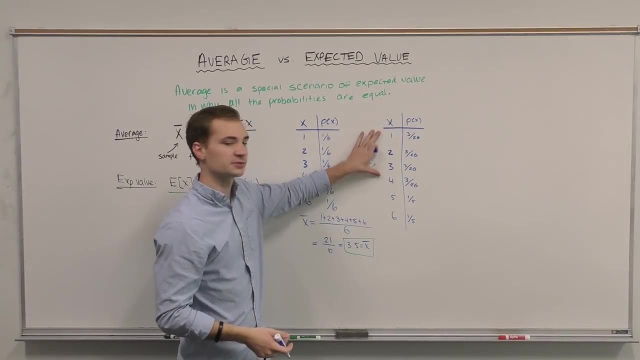 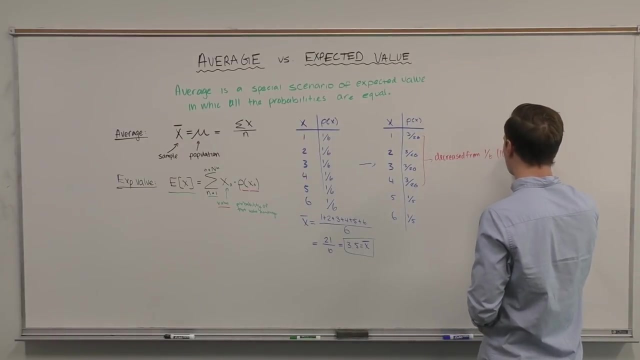 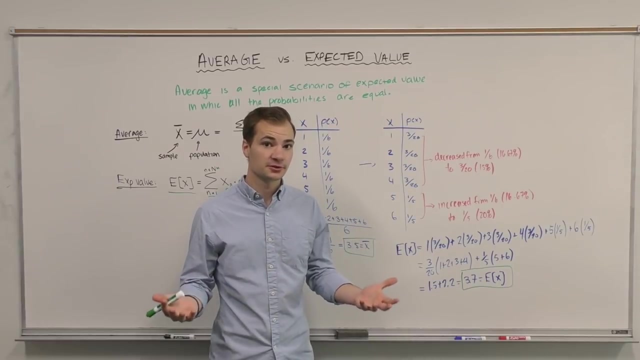 I increased this from a 1 in 6 to a 1 in 5 chance and subsequently lowered the remaining. Now let's look at how this will affect our expected value. We see in this weighted die that our weighted average, which is another word to describe. 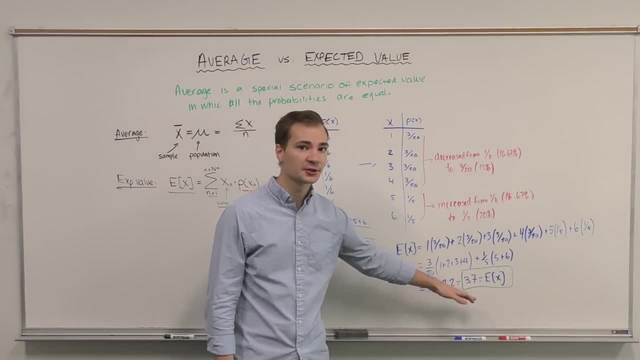 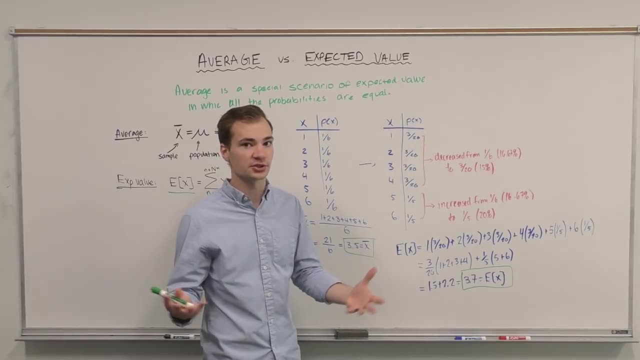 the expected value. Our weighted average is higher Because I'm more likely to roll a 5 or a 6. So this skews my statistic, skews my distribution, if you will- toward a higher value compared to 3.5.. 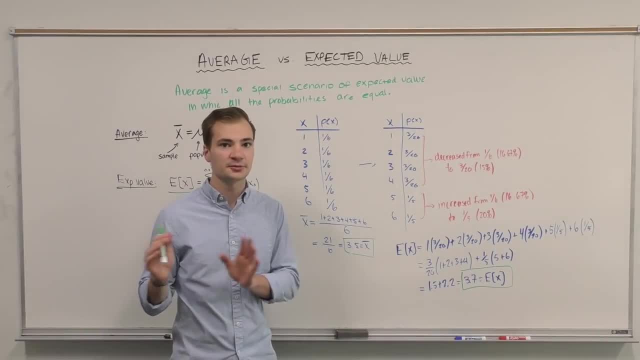 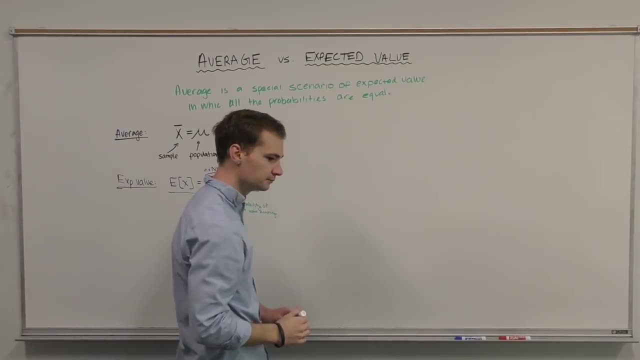 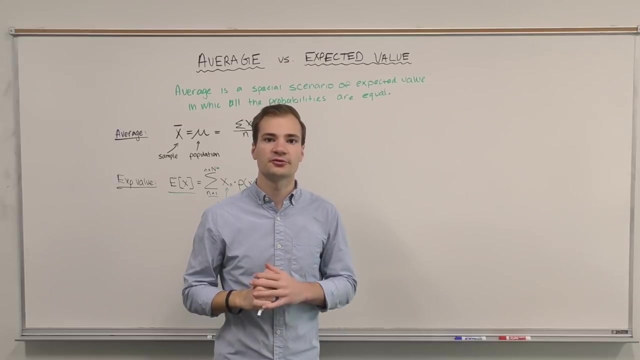 Now let's look at a real world example. that is a little bit outside of probability, but the weighted average still applies. I'm going to set up a scenario where I work two different jobs that earn two different incomes, with two different hours a day. 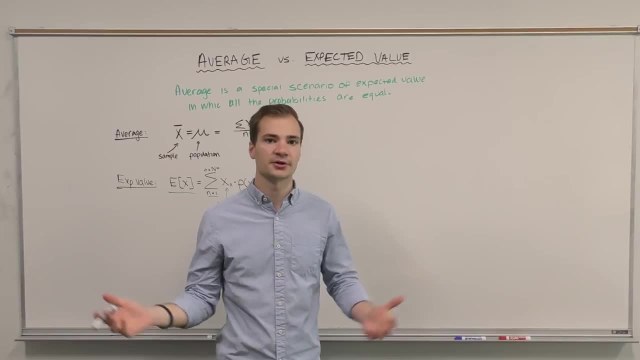 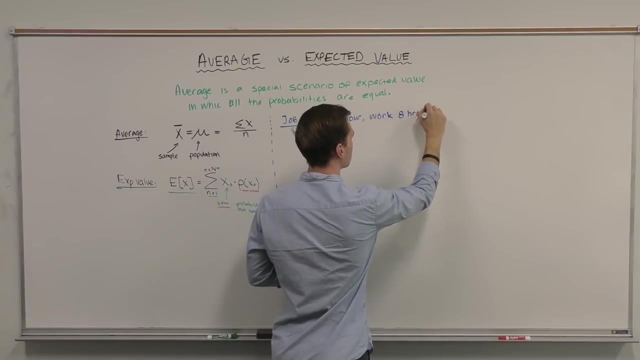 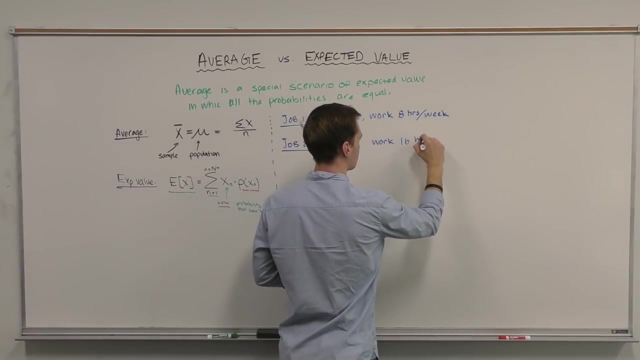 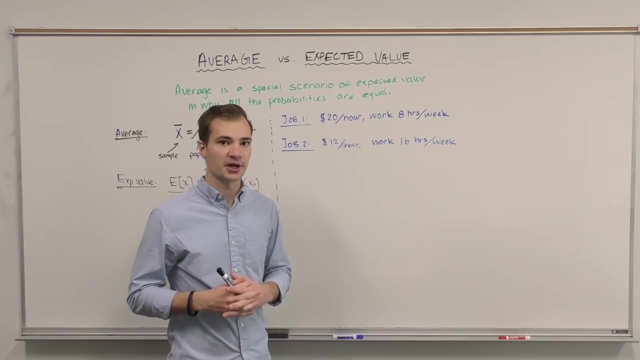 And I want to measure the money that I earn in a given week. Now let's explore the fallacy. if we use the average salary I made, times the number of hours per week. Now let's look at a real world scenario where I work two different jobs that earn two different. 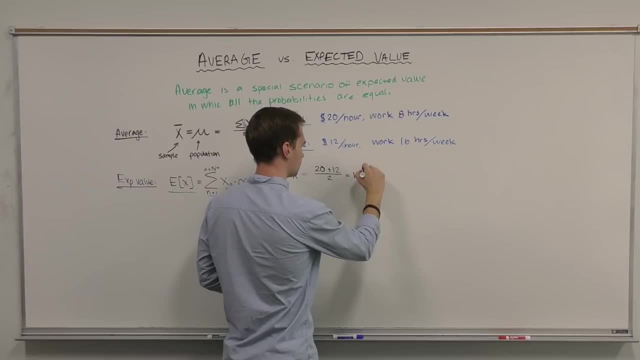 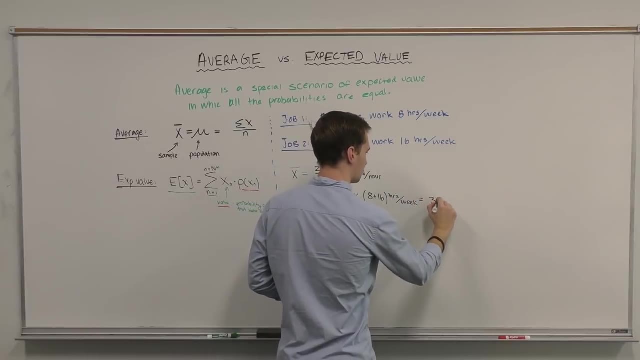 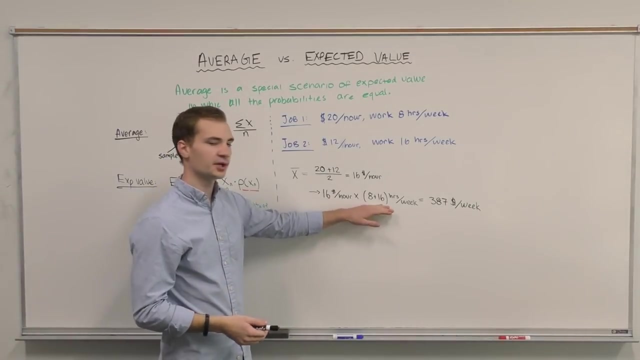 incomes, with two different hours a day And I want to measure the money that I earn in a given week. And I want to measure the money that I earn in a given week. So if I took the average amount I've made with my years and I multiplied that by the 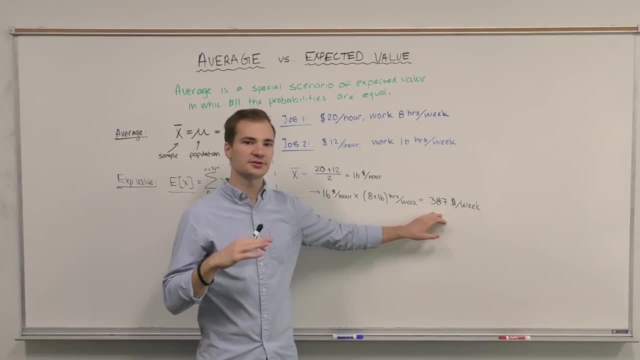 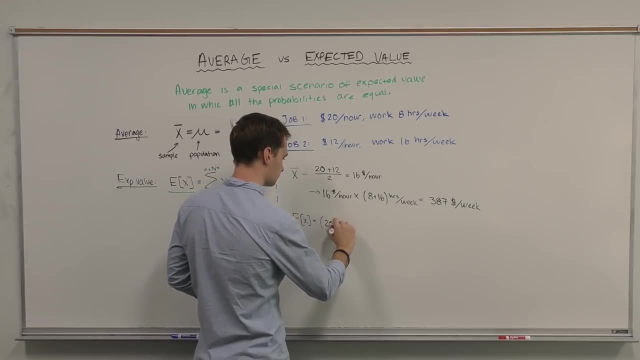 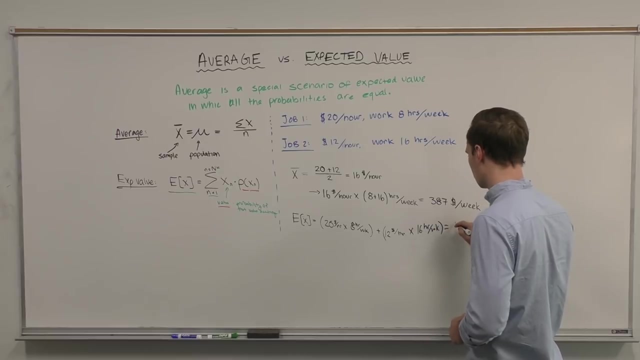 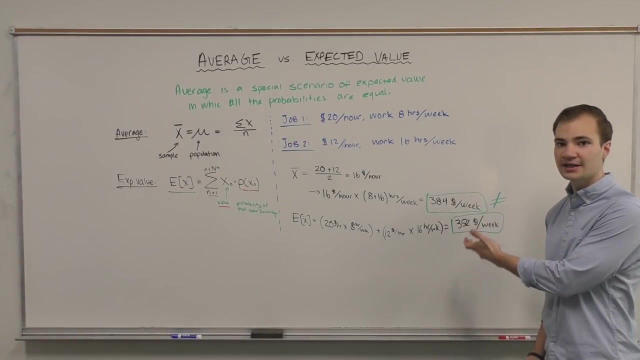 number of hours I work, I'd make $387.. Let's check if this is true or not. No, No, No, For those of you following along, I made two math mistakes And we see that the outcomes of these two are not equal.